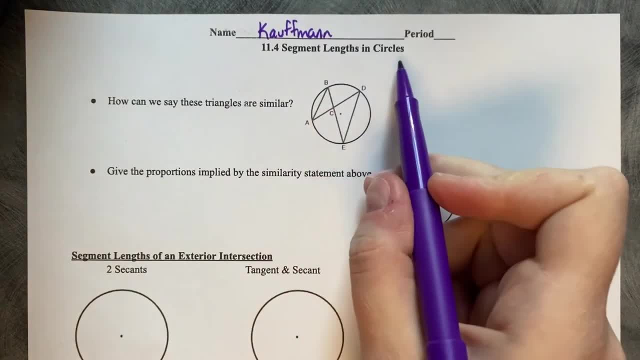 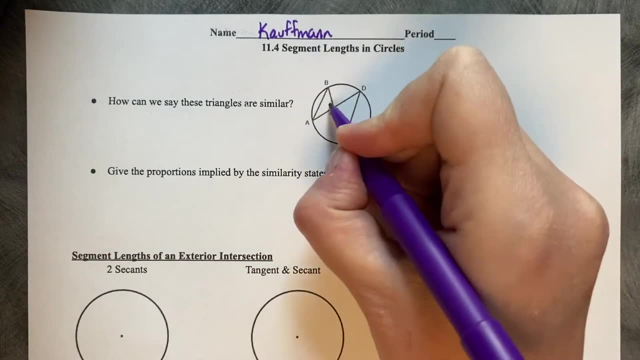 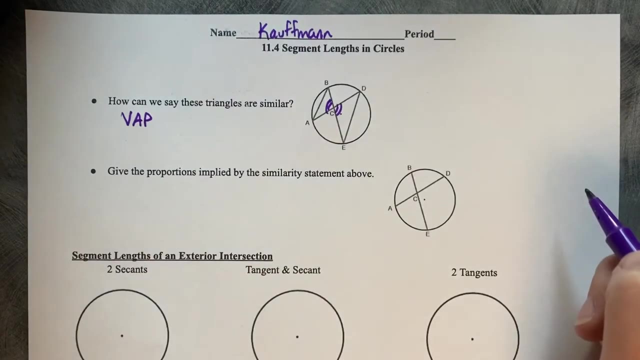 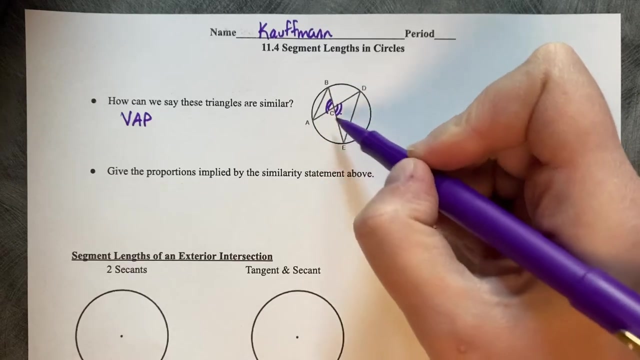 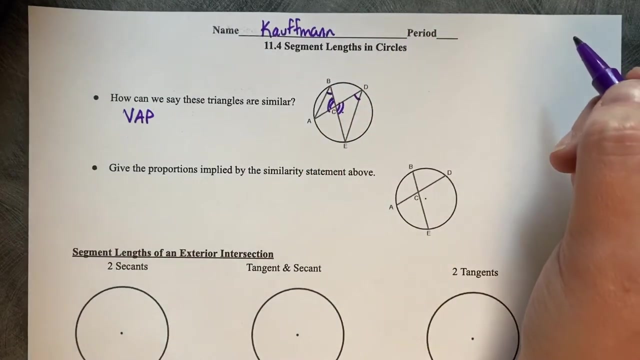 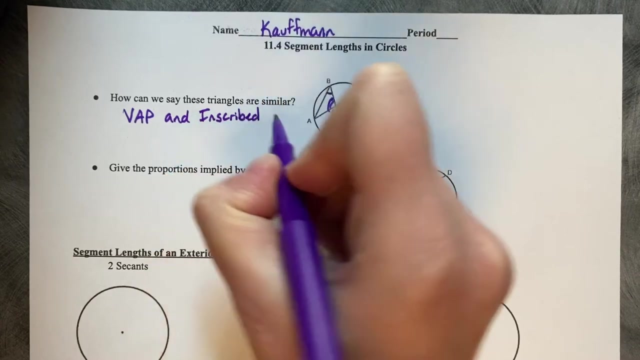 11.4, Segment Lengths and Circles. How can we say that these triangles are similar, These two triangles? Well, first of all, we know that these two angles are vertical angles, so the vertical angles postulate 12.5. Then we can see that the arc AE is shared by both ABE and ADE, which means that angle B at vertex B and angle D are equal angles by the inscribed angles theorem. 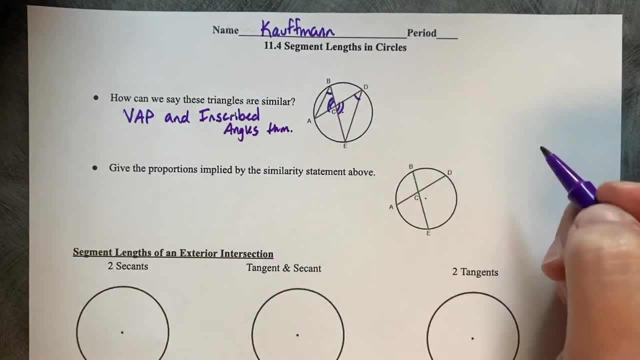 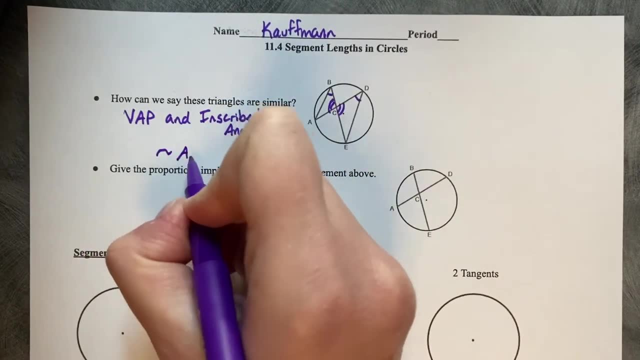 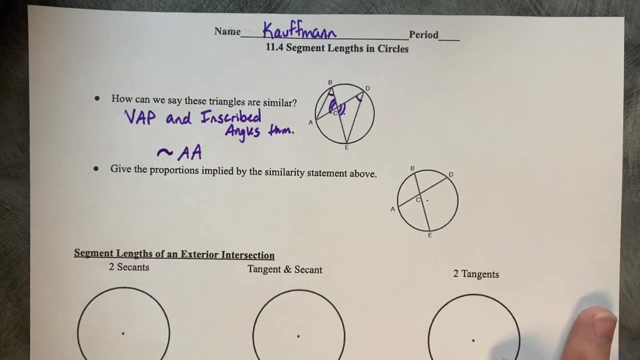 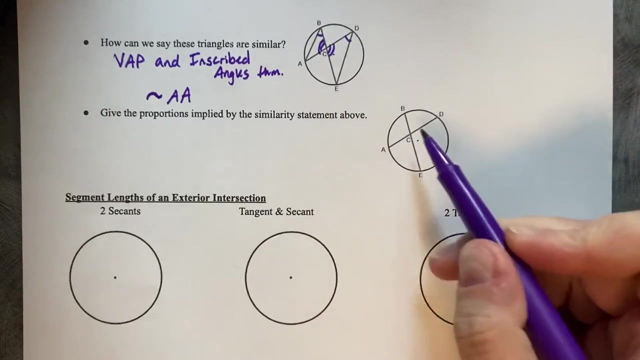 13.5, And to show that two triangles are similar, all you need are two angles- 14.5. So if that's the case, if those two triangles are similar, if I take away the segment ABA and DE, we've got just an intersection of lines inside of a circle, which means that if those two triangles are similar, then their lengths are also similar to each other. 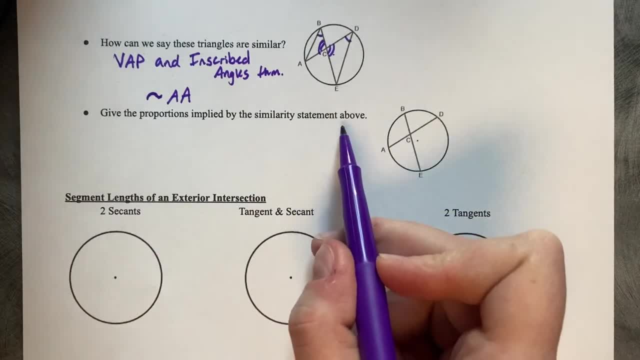 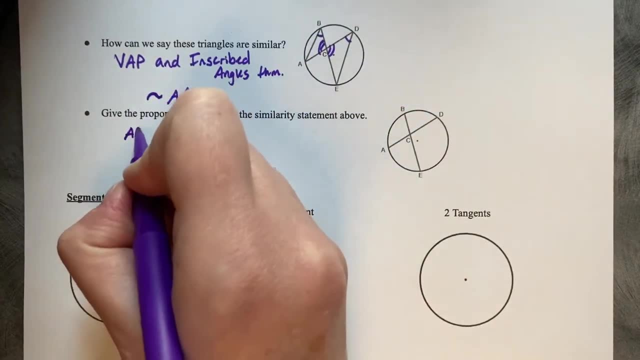 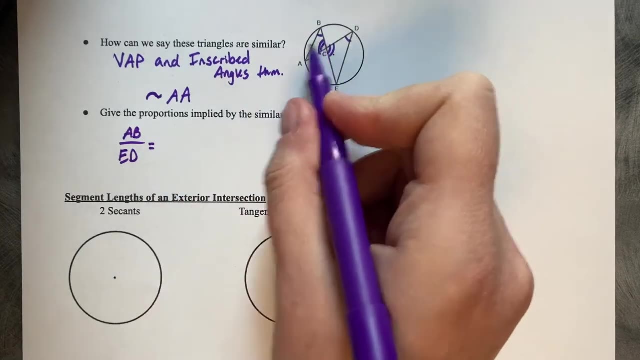 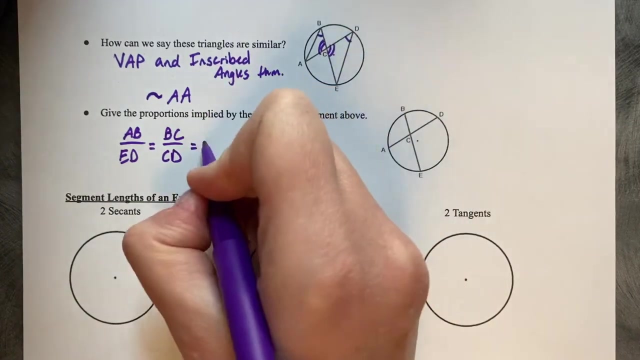 15.6. So give the proportions implied by the segment ABE and ADE, So we can say that AB is similar to ED. 16.5. We can also say that BC is similar to CD and AC is similar to CE. 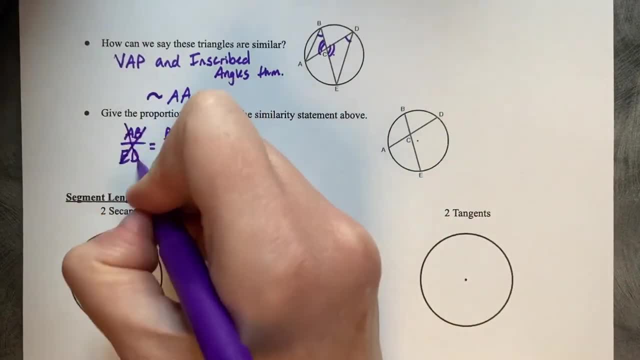 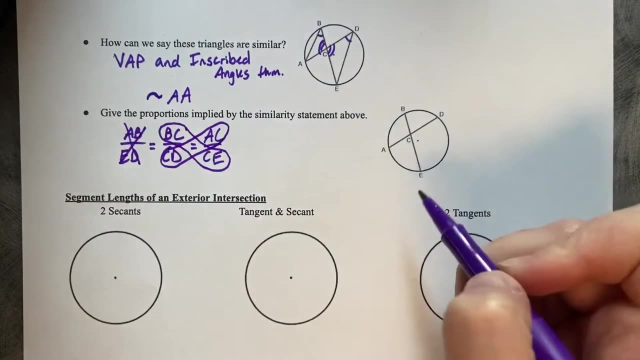 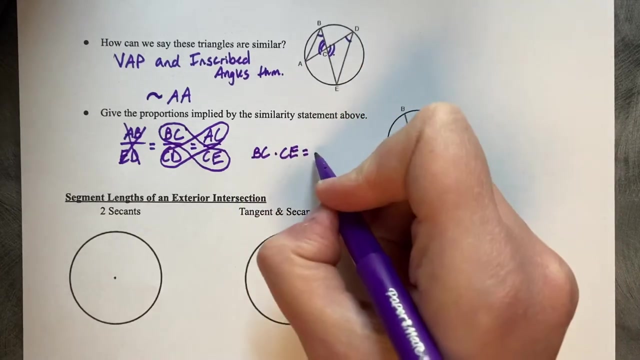 17.5 And then on the diagram you can see we're going to take away those two segments And we're just going to use these two statements to make a linear statement. So we can say that BC times CE is equal to AC times CD. 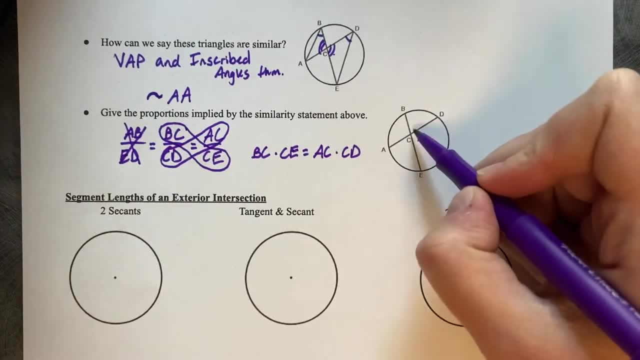 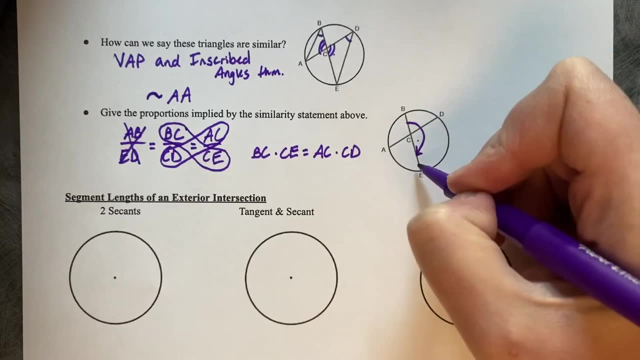 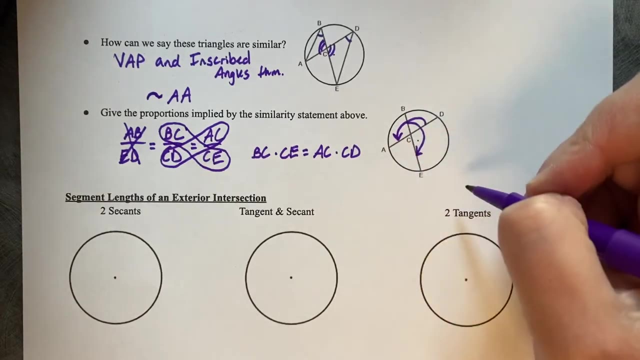 So if we wanted to say they wanted to calculate CD and we knew only the other lengths, you could say BC is times CE and then that's equal to AC times CD. So you're multiplying the two segments together to make your equality statement. 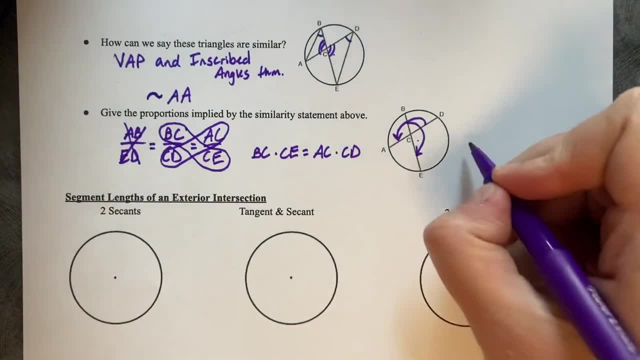 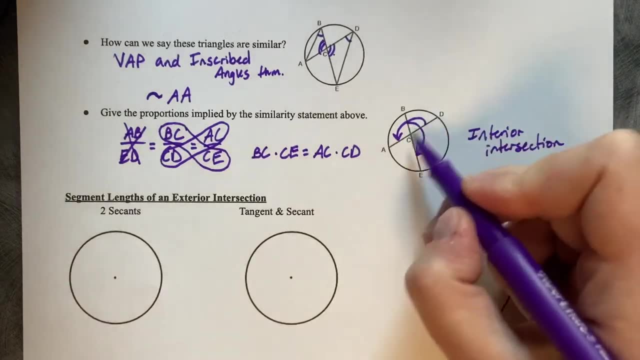 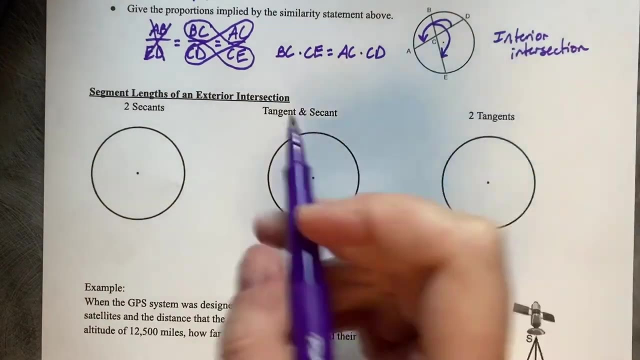 That's for an intersection that's on the inside. This is an interior intersection. You just multiply the two segments together and set them equal, And then we're also going to look. We're going to look at what happens when it's an exterior intersection. 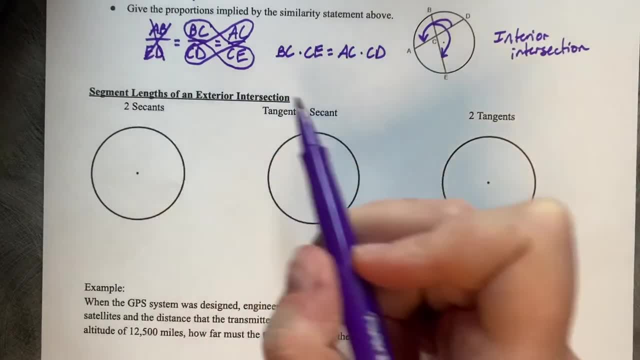 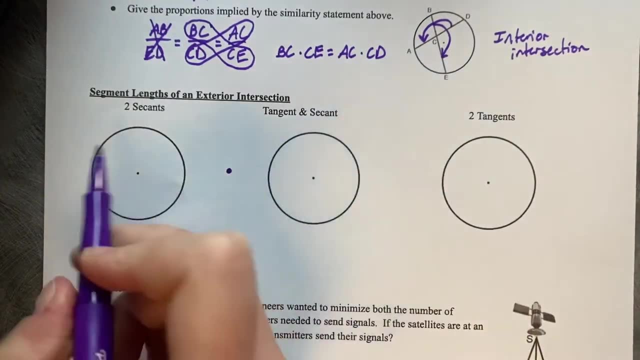 And again there's three different scenarios that can happen: Two secants, a tangent and a secant and two tangents. So let's do two secants first. So let's do an exterior point out here We've got one secant that goes to it and a second secant that goes to it. 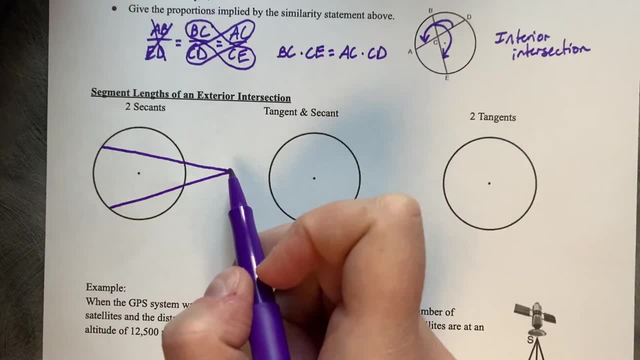 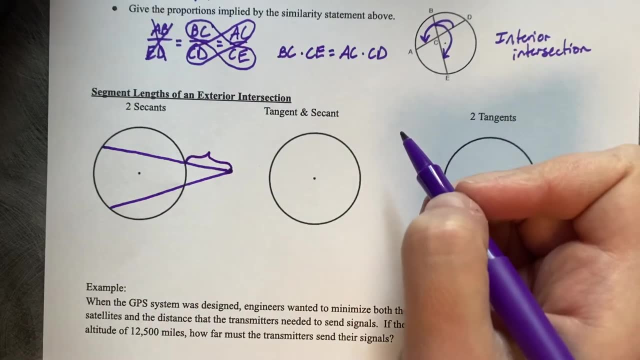 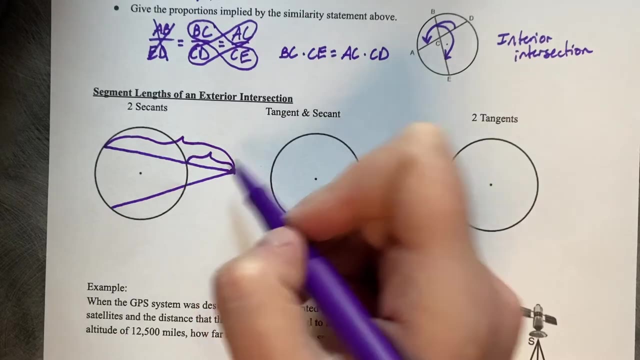 If we want to know something about these lengths. what's happening is that you take this part which is from the edge of the- It's a circle to the intersection, and then you've got this whole segment, And what you do is you multiply those together, similar to this one. 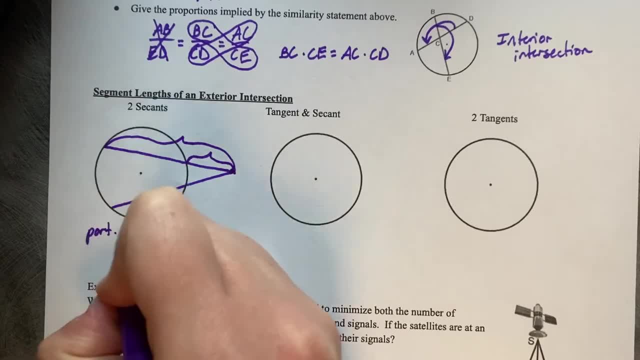 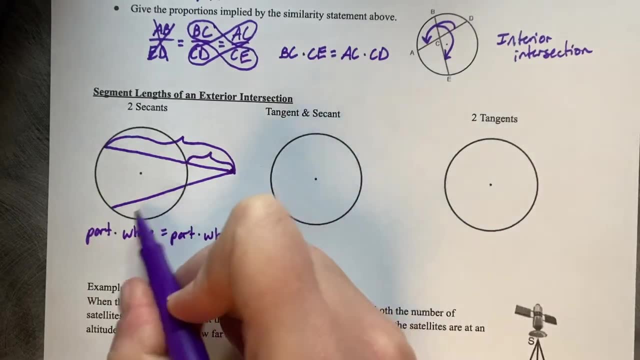 So you're going to- I'm going to just write it out in words- So you're going to do the part times the whole equals the part times the whole of your second segment, of your second secant. How about a tangent and a secant? 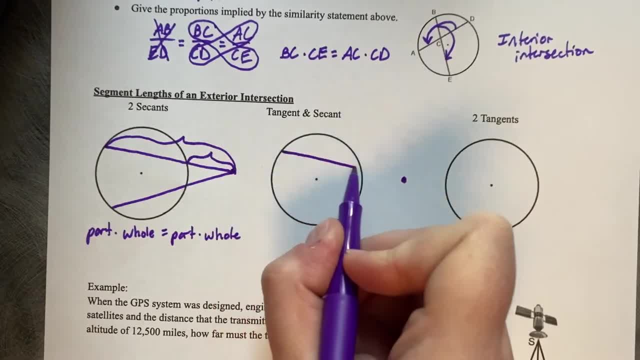 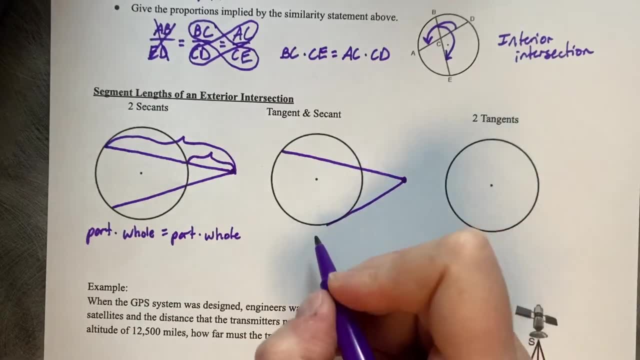 So let's do a similar exterior point. So here's my secant And here's a tangent. So then you would do the part times the whole of your secant, Of the secant P standing for part, And then the tangent. there's no part and whole to it. 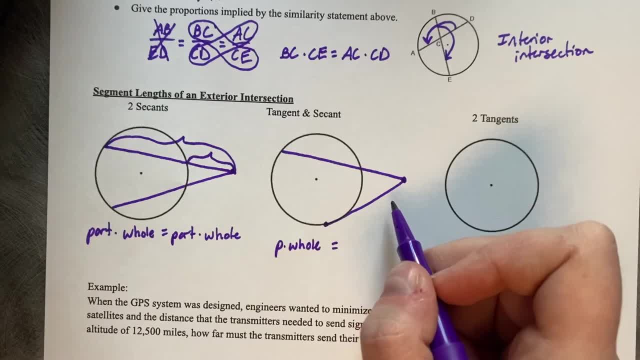 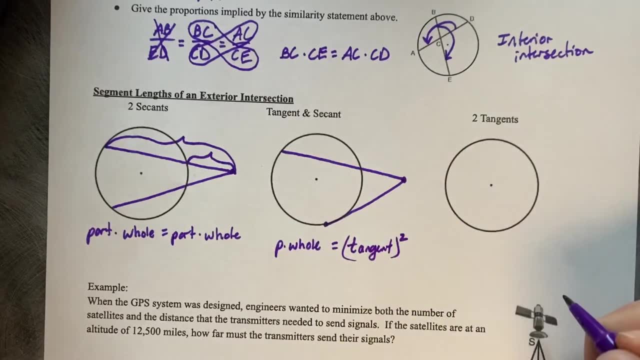 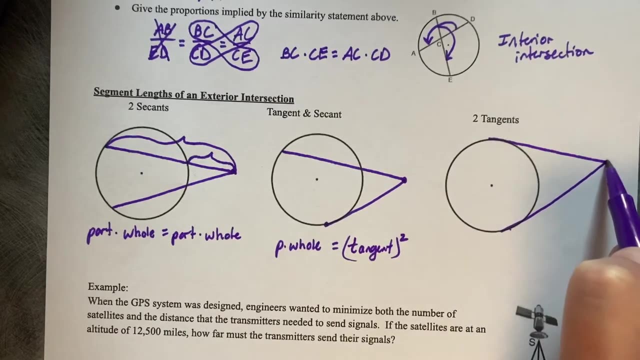 It's just one segment, So you're multiplying it by itself, So it's a tangent times a tangent, Or in other words the tangent squared, Then two tangents, So those two are equal, And it's just going to be a tangent equals a tangent. 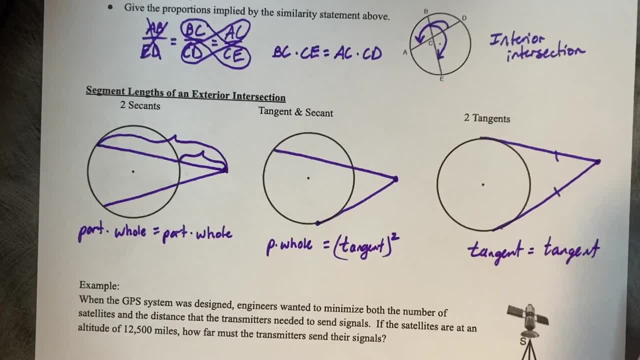 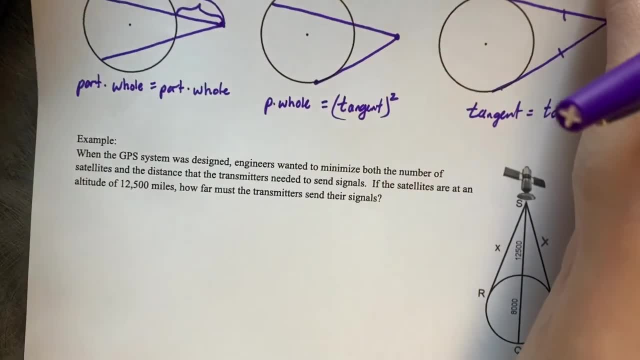 Of course you could do tangent squared equals tangent squared, but that's just more work. We know that those are the same length And we're talking segment lengths today. So here's our example. When the GPS system was designed, engineers wanted to minimize both the number of satellites. 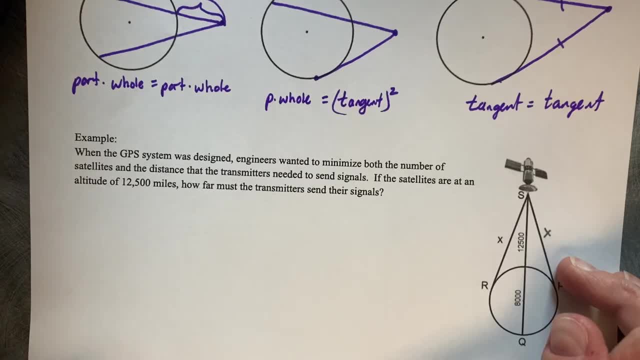 and the distance that the transmitters needed to send signals. If the satellites are at an altitude of 12,500 miles, how far must the transmitters send the signal? So we're looking for this length X, We've got 12,500 to the Earth. 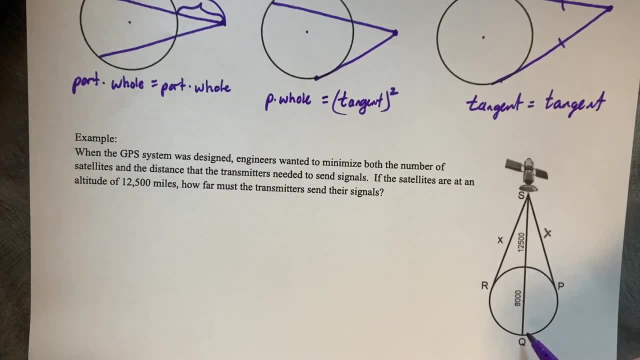 And then we also know that the Earth's diameter is 8,000.. So if you are going to set this up, we want the length of these tangents. This is what's going on, So we're going to be using this second tangent and a secant. 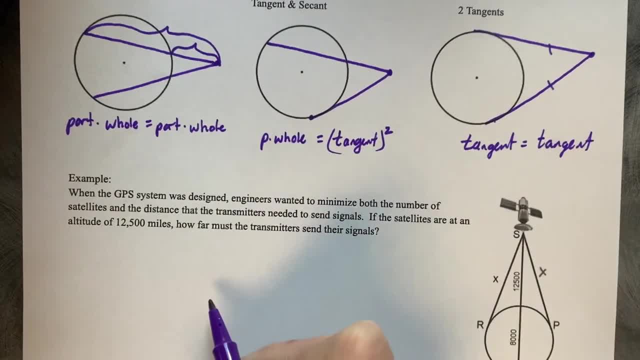 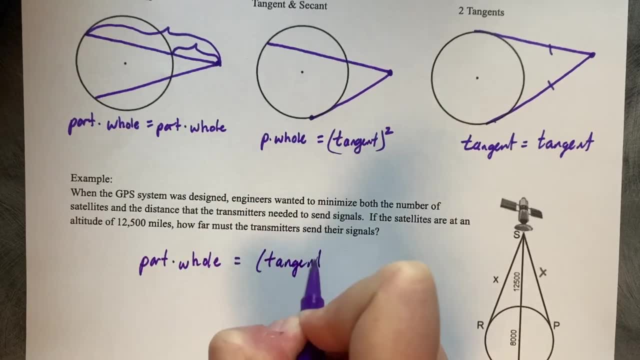 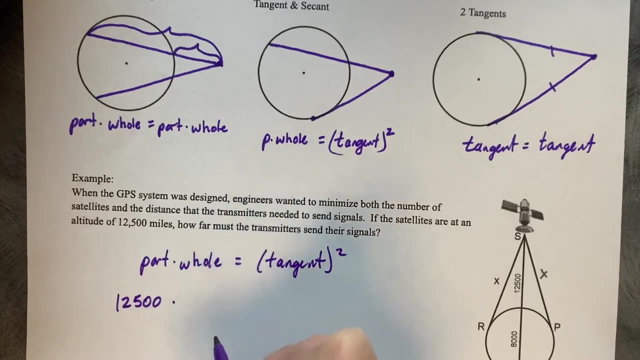 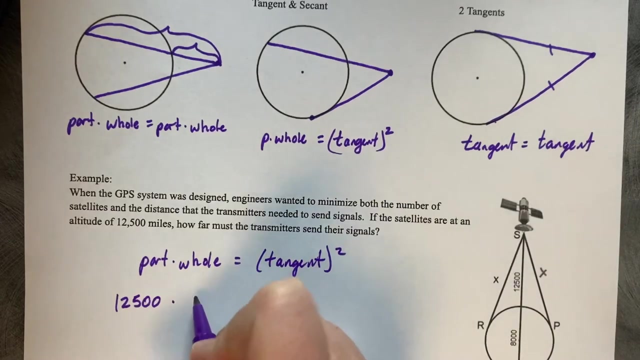 because we've got our secant and a tangent going on. So it's going to be a part times a whole equals the tangent squared. So that's going to be 12,500.. That's our part Times our whole. 12,500 and 8,000 is 22,000.. 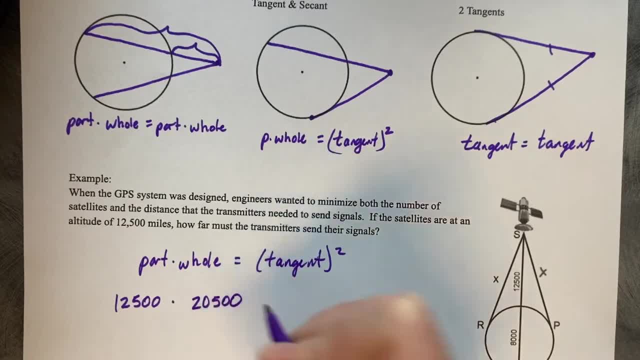 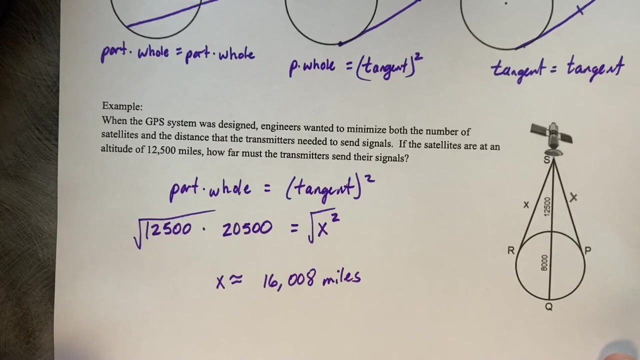 20,500 equals our tangent squared, and that's a missing piece. so X squared. Multiply that and then take the square root, and X is approximately 16,008 miles long. Sorry, you couldn't see that. All right, let's check up with some naked number problems here. 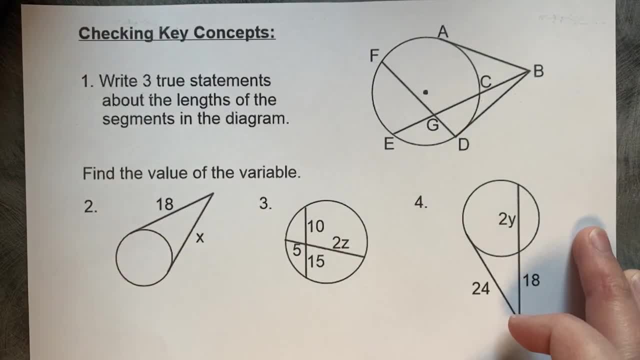 checking key Et. we're still looking at the argument. If we look at the constant, we know that the constant is going to be zero. So we want to assess that And we're going to take this function, the EG, and for this we're going to use the binary order. 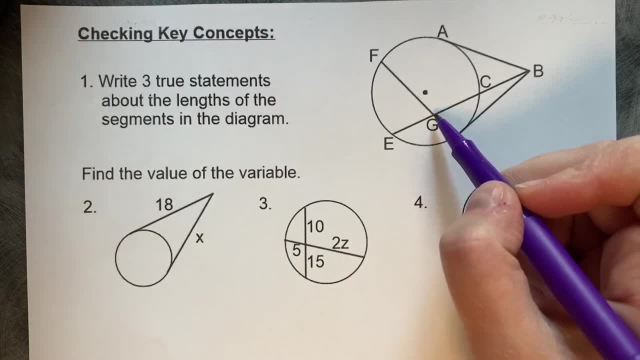 So we're going to use this function and we're going to apply that to our answer, And we're going to use it to deduce that our answer is positive, Because we're also going to have a lot of arguments where the problem is going to be positive. 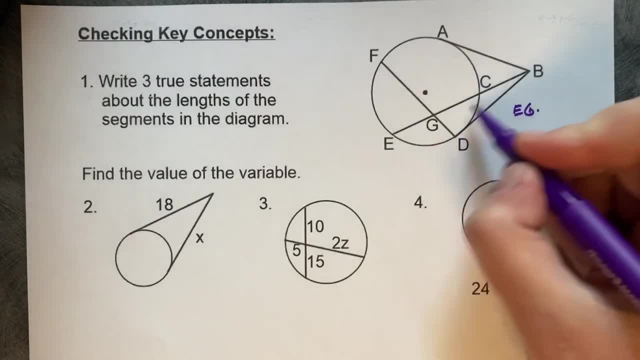 but just not that we're going to get a positive answer. So that's why we're going to use this result here, And then we're going to take this power factor and we're going to use the same equation to measure out the difference between our values. 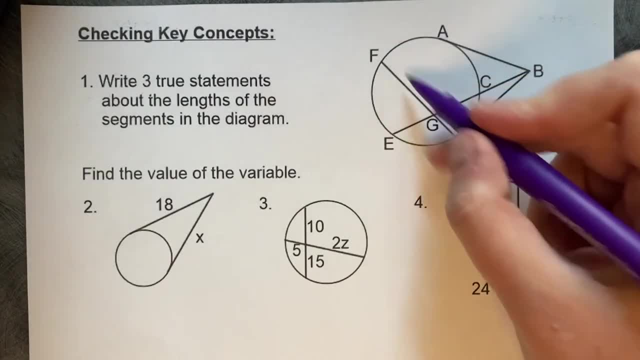 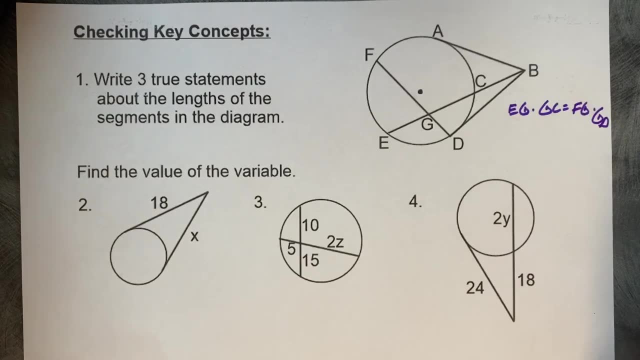 So, if I have the same answer here- is equal to FG times, GD. Sorry, that's running off the page there. Okay, I see two tangents. We can say that AB is equal to BC- I'm sorry, BD, Those are congruent.